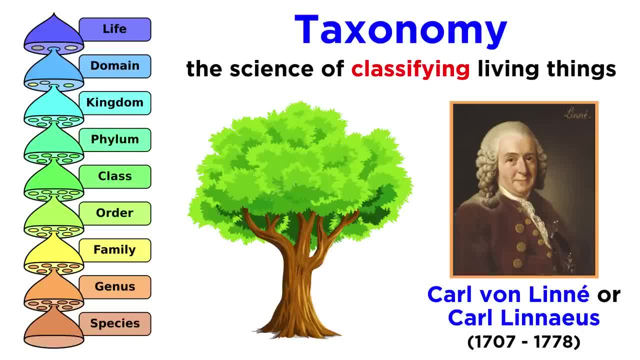 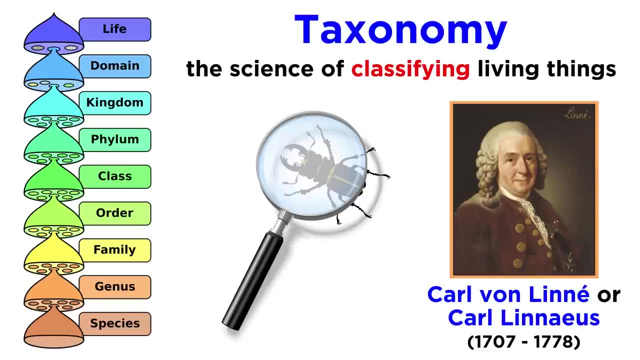 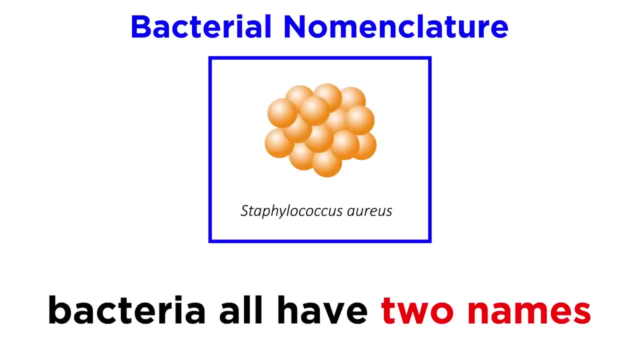 ever since Swedish botanist Carl von Linnaeus, also called Linnaeus, established a system for classification. He wanted to minimize chaos as new species were discovered and provide a structure for defining and recognizing any newly discovered species. In the case of bacteria, we use a binomial or two-name system of nomenclature. 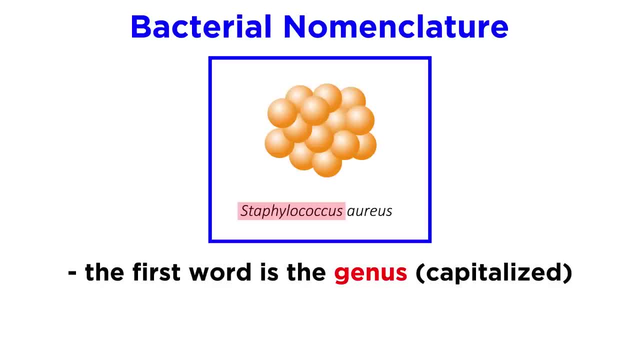 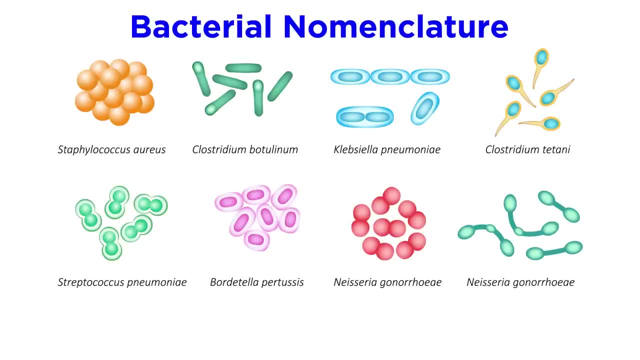 The scientific name for any bacteria is always the name of the genus first, which is capitalized, followed by the species name. Both should be italicized. The names of the genus and species have a wide variety of origins. Sometimes they were named after the microbiologist that discovered them. 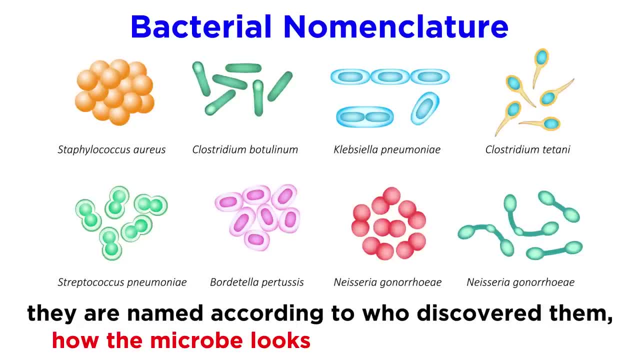 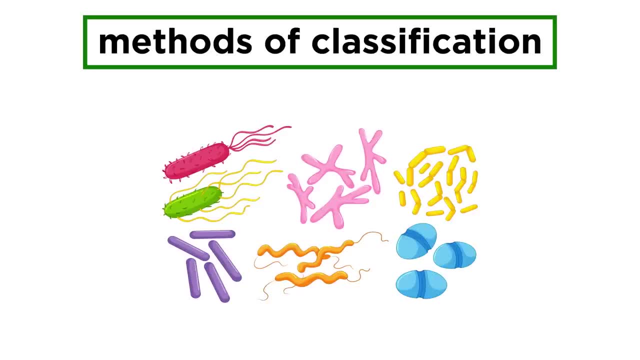 In other cases, the name might be related to how the microbe looks or the disease it causes. Now that we've covered the names, let's talk about how bacteria got sorted into the into their respective categories in the first place. When it comes to classifying bacteria, it may seem a daunting or even impossible task. 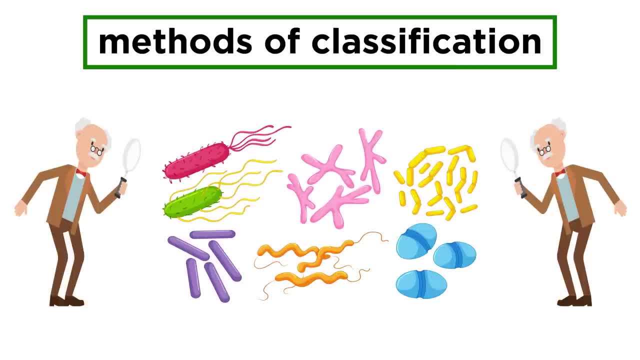 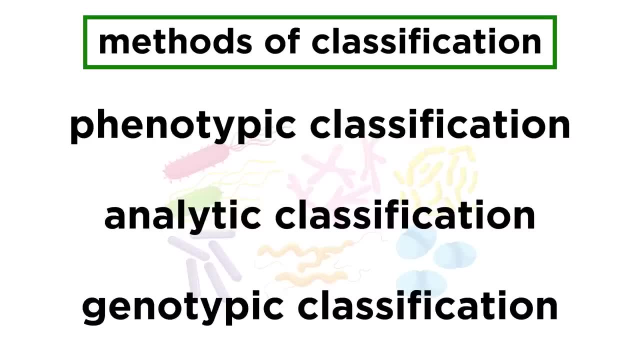 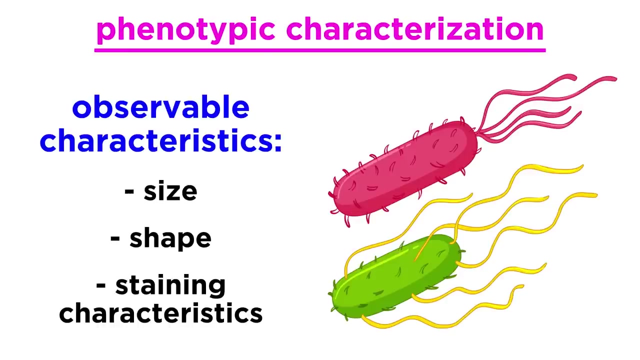 However, scientists have developed a system to observe, test and then categorize bacteria into logical relationships. There are three main types of classification: phenotypic, analytic and genotypic. Let's talk about what each of these are. First, let's talk about phenotypic characterization, meaning the set of observable characteristics. 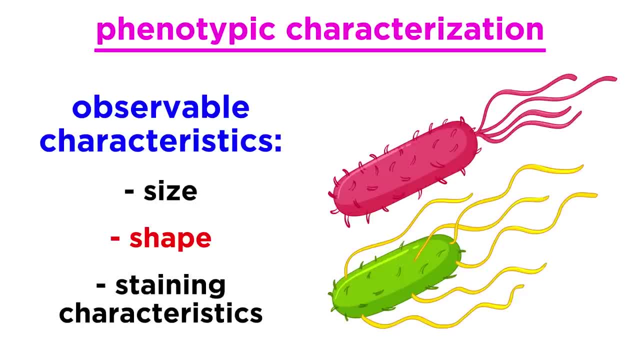 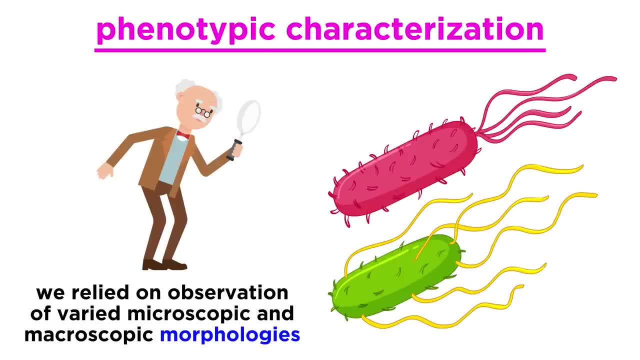 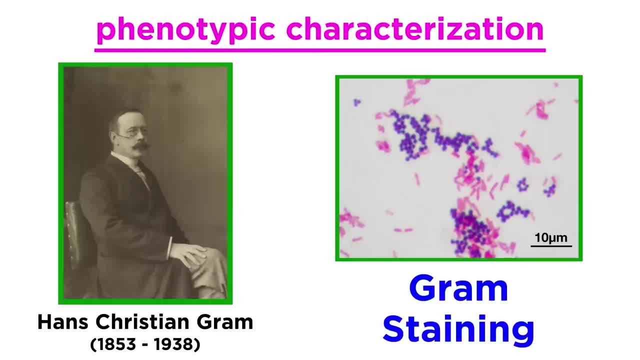 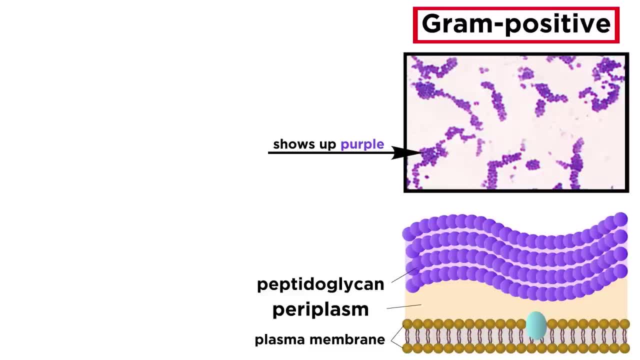 their cell wall contains Gram-positive organisms have a thick peptidoglycan wall retaining lots of crystal violet stain when using this method and thus appearing a vivid blue under a microbe. That's the way the method works: microscope. 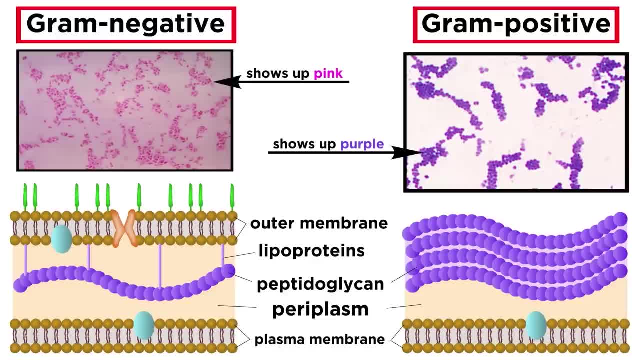 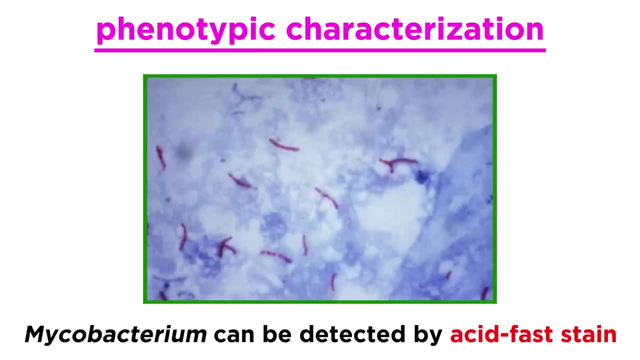 Gram-negative organisms have a much thinner peptidoglycan layer which does not hold the blue dye. Even just separating bacteria into gram-positive versus gram-negative can tell us a lot about how they might behave. Certain microbes have unique staining characteristics, such as the genus Mycobacterium, which can. 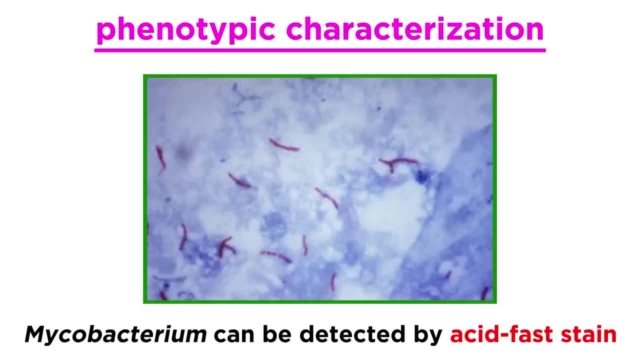 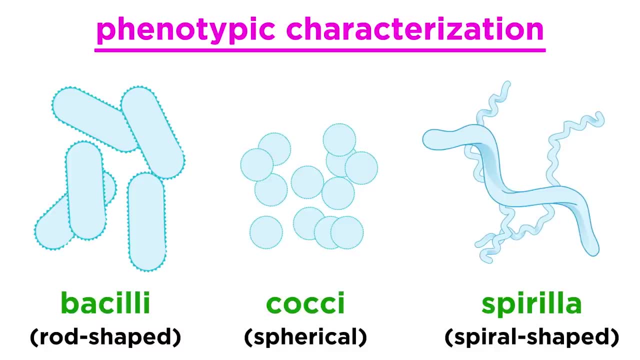 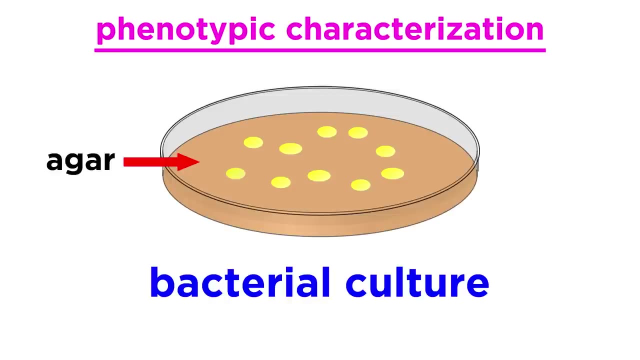 be detected by an acid-fast stain. Another example involves identifying the shape of individual organisms under a microscope, which will be either rods, cocci, curved or spiral. Zooming out a bit, scientists also look at how bacteria grow on agar in the lab. 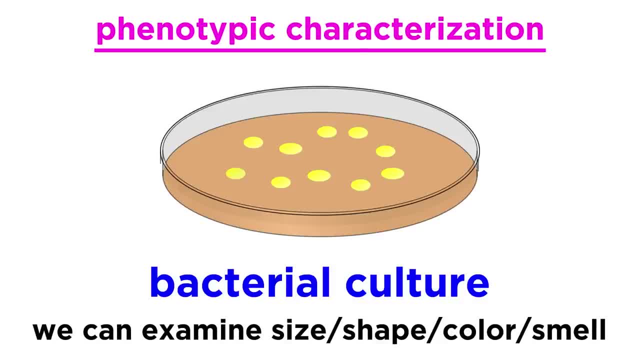 They look at the colonies of bacteria that grow, taking note of the size, shape, color and even smell. For instance, streptococci colonies tend to be small. They tend to be smaller in relation to most other types of bacteria and serratia marcescens. 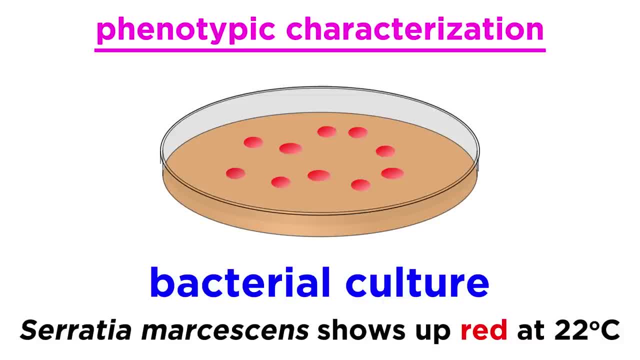 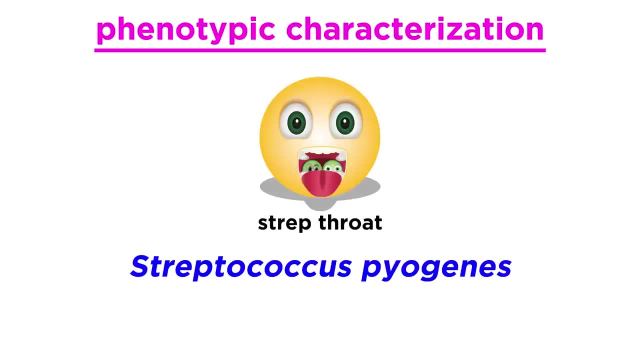 typically appear red when grown at 22 degrees Celsius. We can test for hemolytic properties on blood agar, identifying if the bacteria produce toxic byproducts capable of destroying red blood cells. For example, Streptococcus pyogenes, the causative agent of strep throat, is a gram-positive. 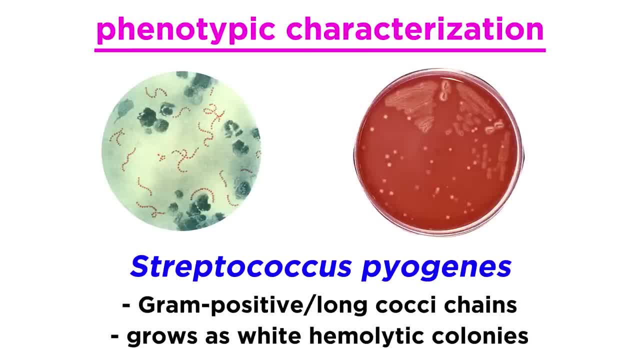 bacterium that forms long-term. It forms long cocci chains and grows as small white hemolytic colonies on blood agar plates. Since it is likely for multiple species to appear similar in these types of tests, these phenotypic characterization methods serve only as a starting point for further investigation. 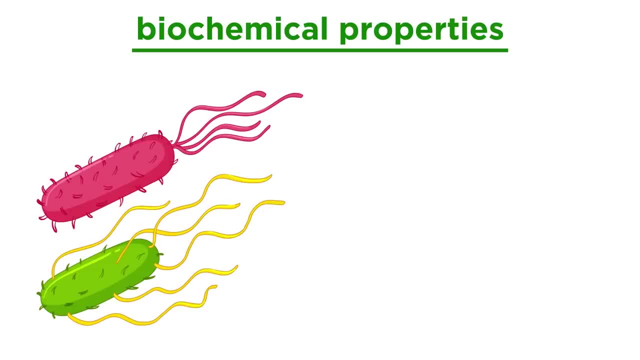 Next, there are tests to determine what biochemical properties the bacteria have, like the ability to ferment specific carbohydrates, What carbon sources they can use for growth, And the presence or absence of different enzymes like lipases, proteases or nucleases. 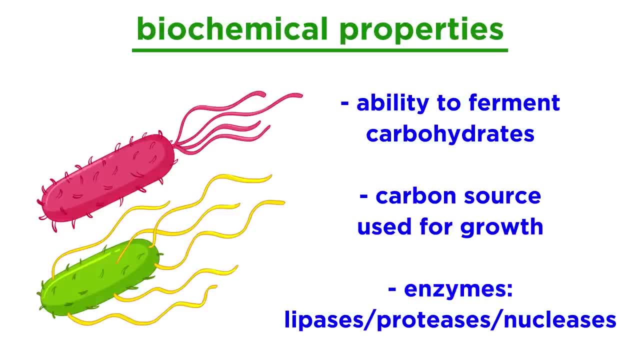 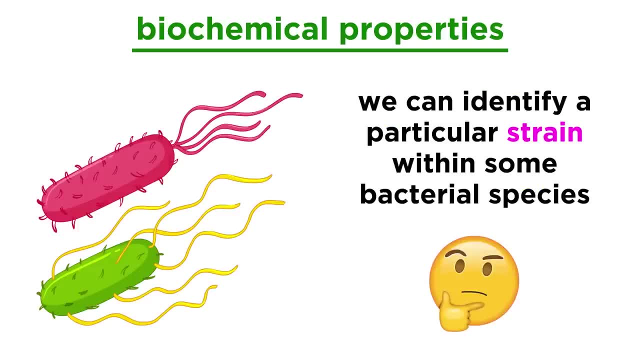 All of these observations combined can identify with reasonable precision a species of bacteria. These techniques have also been used to subdivide groups of organisms beyond the species level down to a specific strain, Doing this by looking at the genetic makeup of the organism, especially in the case of 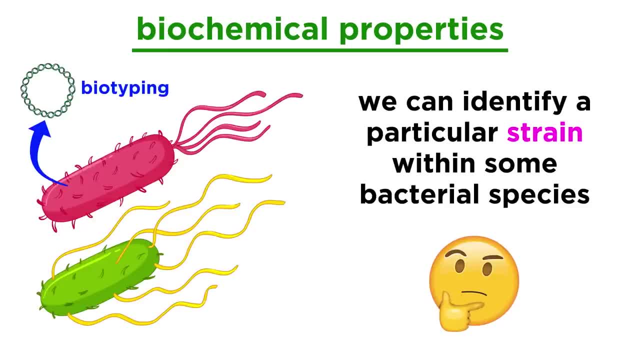 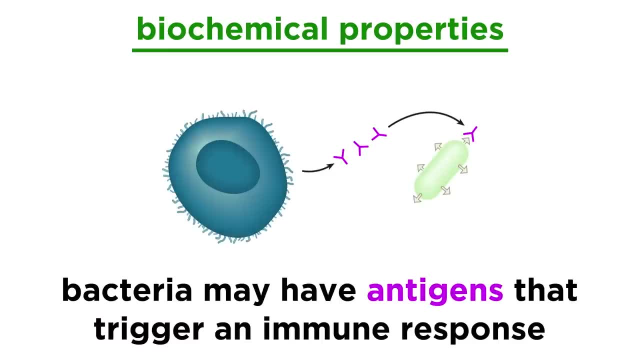 an outbreak is called biotyping. Many bacteria also possess antigens which might be a toxin or other substance that triggers an immune response in the body. Grouping bacteria based on these antigens is called serotyping. Using serotyping, scientists can work backwards using antibodies which can be found in the 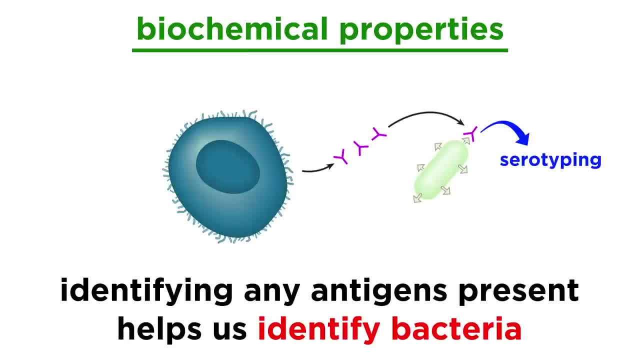 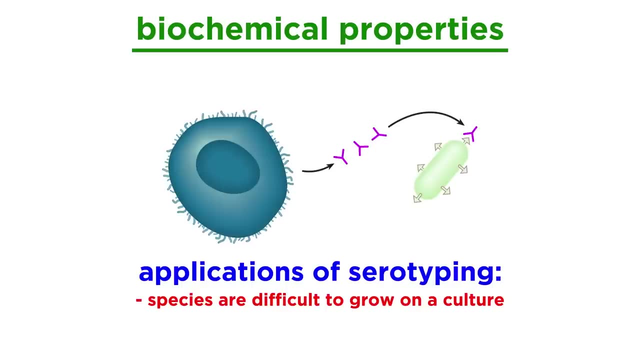 body. This allows scientists to detect which antigens are present, thus allowing them to narrow down the bacterial possibilities. Serotyping is a powerful tool for classification, especially for those species that are difficult to grow, those that are difficult to test biochemically or those that need to be identified. 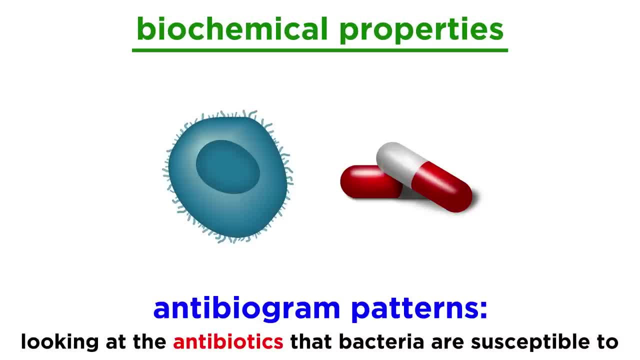 rapidly, such as during an outbreak. Scientists can also look at which antibiotics bacteria are susceptible to. For example, if you have a bacteria that is susceptible to an antibiotic, you can look at which antibiotics bacteria are susceptible to. This is called biotyping, which is called analyzing their antibiogram patterns. 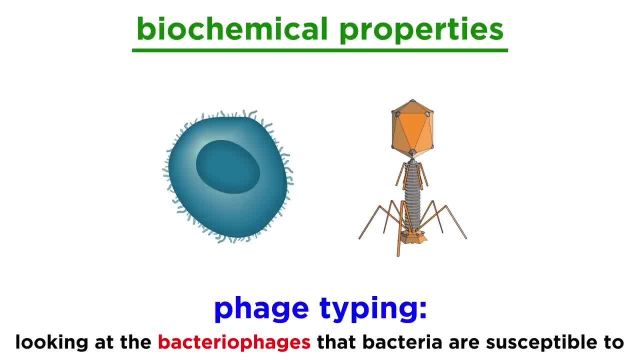 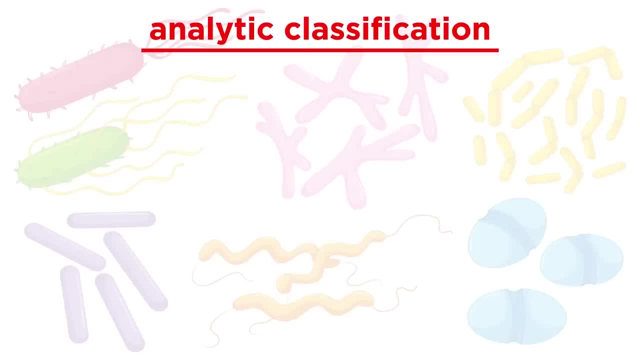 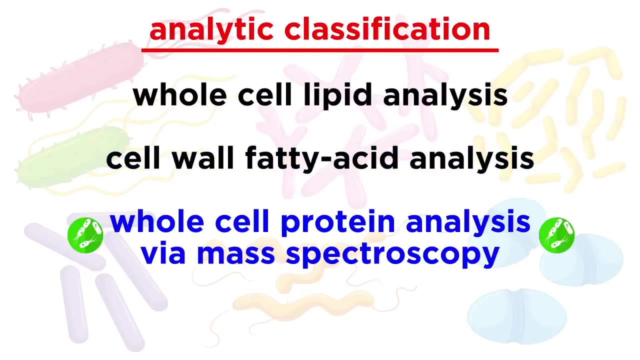 Finally, using phage typing, scientists can assess which bacteriophages bacteria might be susceptible to. Now that we've covered phenotypic classification, let's move on to analytic classification. Analytic classification methods include whole-cell lipid analysis, cell wall fatty acid analysis. 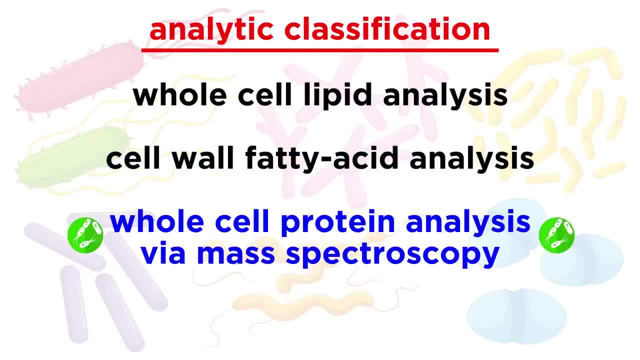 whole-cell protein analysis via mass spectroscopy and the presence of cellular enzymes via multi-locus enzyme electrophoresis. Analytic classification can be a bit labor-intensive, requiring expensive machines and specialized training. For these reasons, analytic classification is typically done in special laboratories. 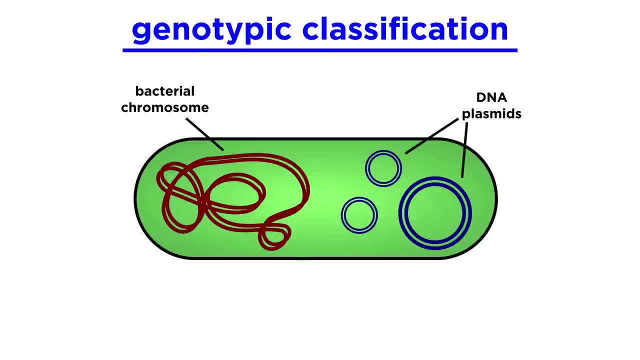 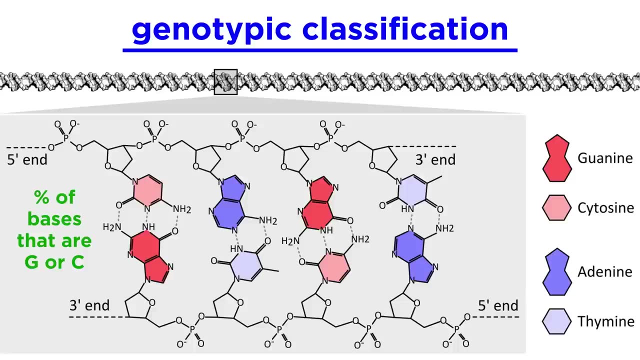 Finally, the most precise method for classifying bacteria is through genotypic classification. Put simply, this means using bacterial DNA to determine what species or family bacteria might belong to. In the early days, scientists used the ratio of guanine and cytosine to classify bacteria. 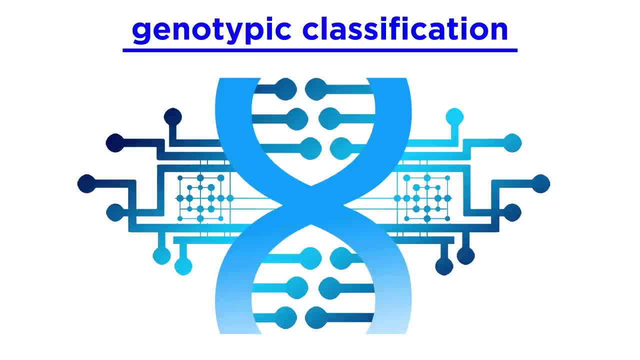 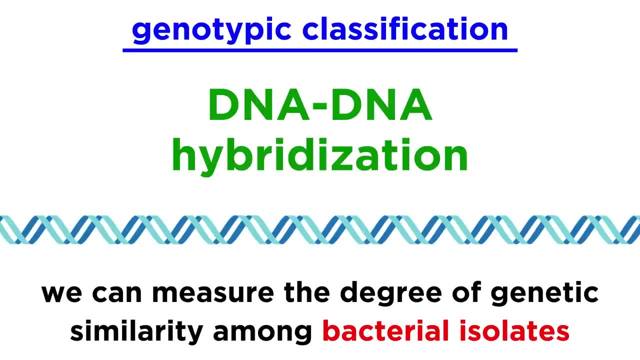 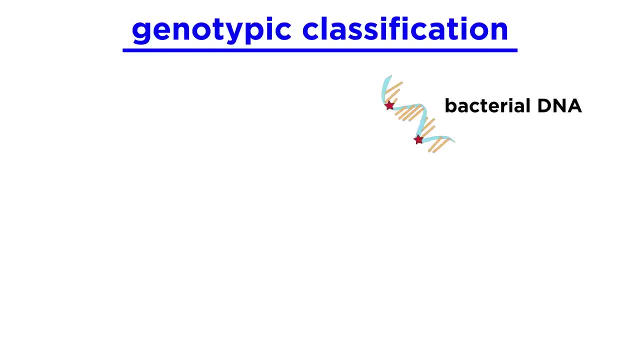 As technology has progressed, so has our ability to quickly and accurately identify bacteria using DNA. Using DNA-DNA hybridization, scientists measure the degree of genetic similarity among bacterial isolates. Taking this a step further, scientists can extract DNA from an organism and expose it. 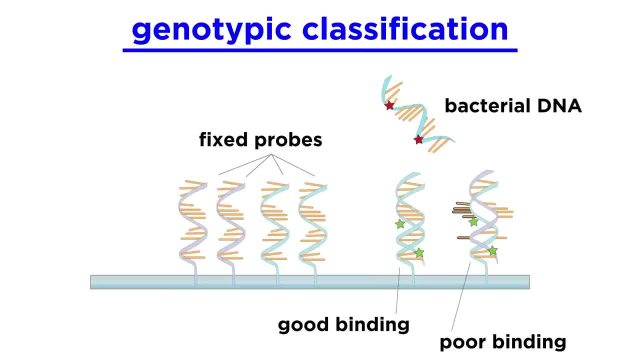 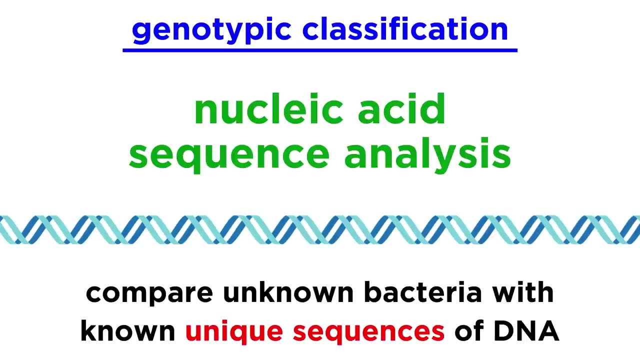 to species-specific molecular probes. If the nucleic acid probe binds to the DNA, then you know you've properly identified the organism. We can also use nucleic acid sequence analysis to compare unknown bacteria with already-known sequences that are unique to a genus, species or subspecies. 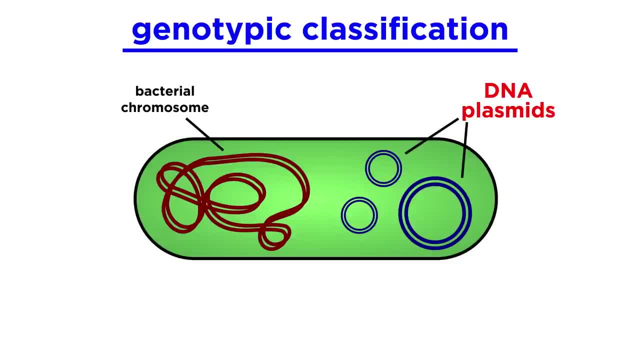 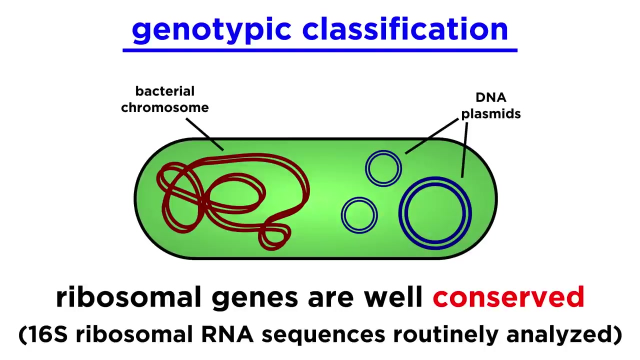 Additionally, some bacteria carry plasmids, which are small circular DNA strands that replicate independently of the chromosome. And while the genetic makeup of bacteria can vary drastically between species, their ribosomes, their ribosomal genes, are remarkably well conserved. Scientists routinely use 16S ribosomal RNA sequences to establish taxonomic relationships. 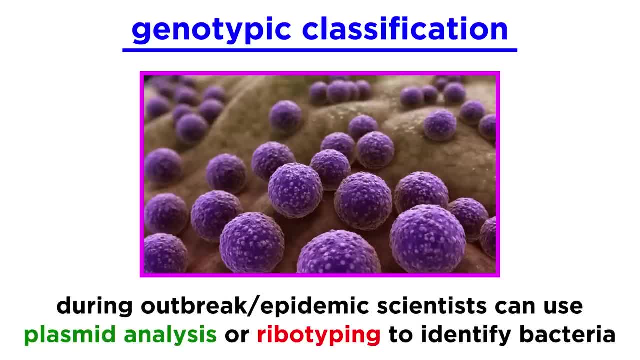 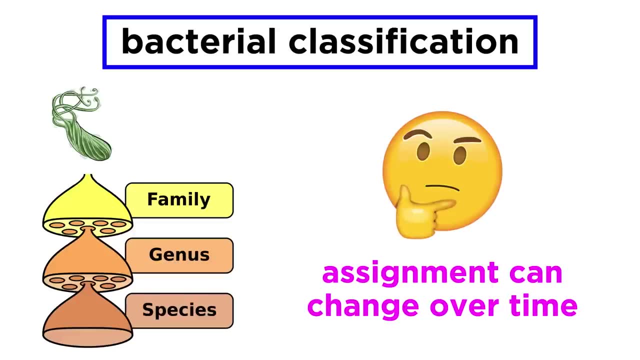 between prokaryotic strains. That's why, in situations such as an outbreak or epidemiological investigation, scientists can use plasmid analysis or ribotyping to quickly identify bacteria. Now here's the thing: Bacterial classification into families, genera and species changes all the time, evolving.